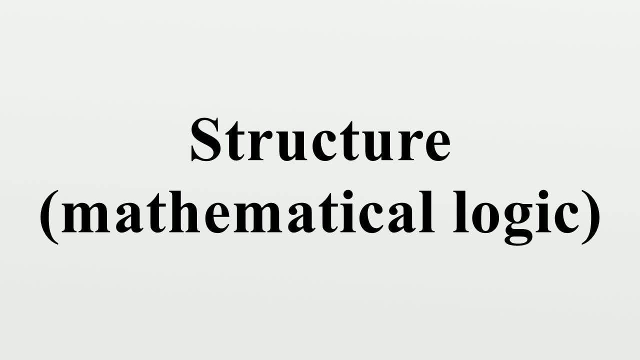 of that theory, Although it is sometimes disambiguated as a semantic model when one discovers that a structure possesses the notion. in the more general setting of mathematical models, Logicians sometimes refer to structures as interpretations. In database theory, structures with no functions are studied as models for relational databases. 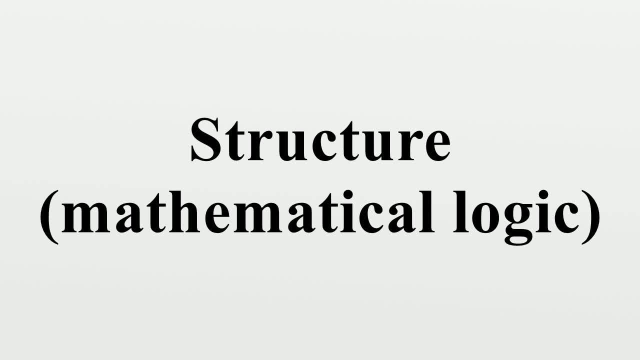 in the form of relational models. Definition: Formally, a structure can be defined as a triple consisting of a domain A, a signature sigma and an interpretation function I. that indicates how the signature is defined To be interpreted on the domain. To indicate that a structure has a particular signature sigma, one can refer to it as a sigma structure. 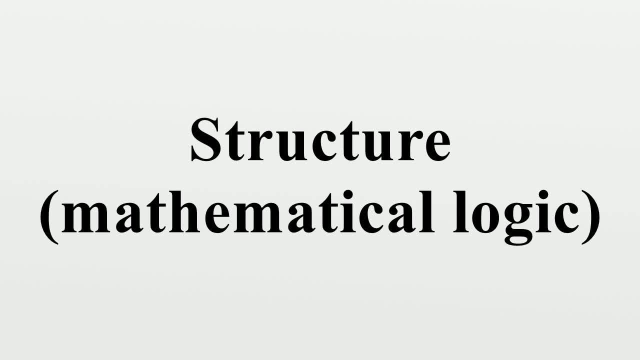 Domain, The domain of a structure is an arbitrary set. It is also called the underlying set of the structure, its carrier or its universe. In classical first-order logic, the definition of a structure prohibits the empty domain. Sometimes the notation or is used for the domain of. 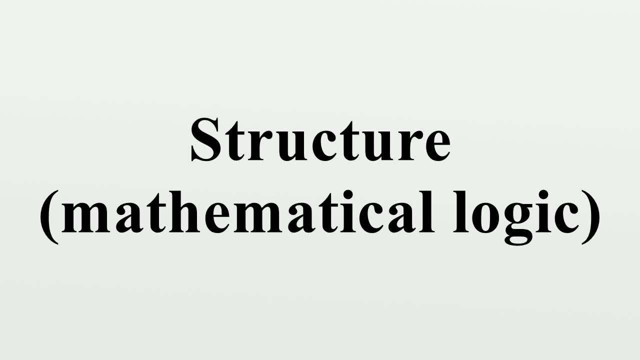 but often no notational distinction. The definition is made between a structure and its domain Signature. The signature of a structure consists of a set of function symbols and relation symbols, along with a function that ascribes to each symbol s a natural number, which is called the arity of s, because it is the arity of the interpretation of s. 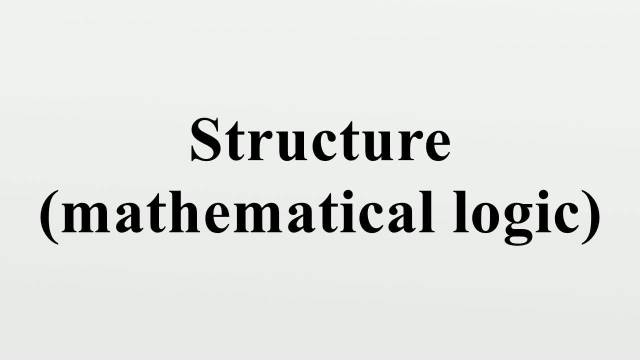 Since the signatures that arise in algebra often contain only function symbols, a signature with no relation symbols is called an algebraic signature. structure with such a signature is also called an algebra. This should not be confused with the notion of an algebra over a field Interpretation function. 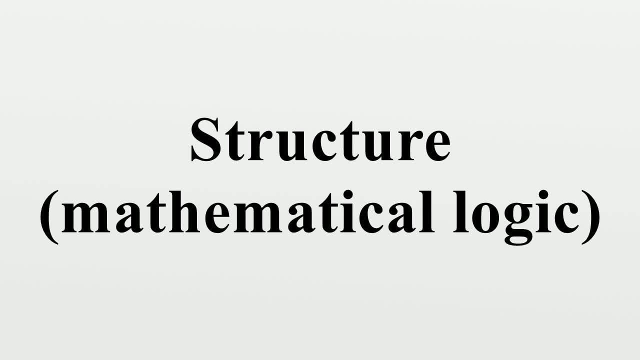 The interpretation function I of assigns functions and relations to the symbols of the signature. Each function- symbol f of arity n is assigned an nary function on the domain. Each relation- symbol r of arity n is assigned an nary relation on the domain A nary function. symbol c is called a constant symbol because its 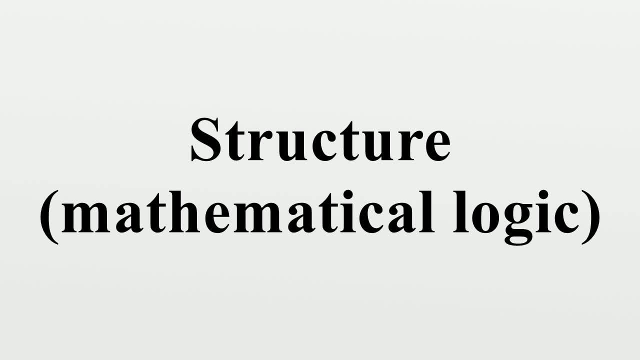 interpretation. I can be identified with a constant element of the domain. When a structure is given by context, no notational distinction is made between a symbol s and its interpretation. I, For example, if f is a binary function symbol of one, simply writes, rather than examples, the standard signature sigma f. 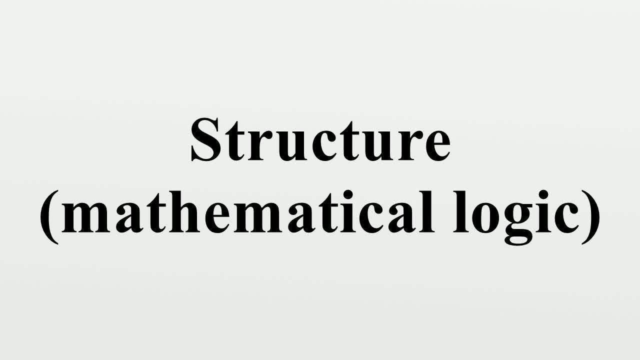 for fields consists of two binary function symbols- Symbols plus and times, a unary function symbol minus, and the two constant symbols zero and one. Thus, a structure for this signature consists of a set of elements, a, together with two binary functions, a unary function and two distinguished elements. 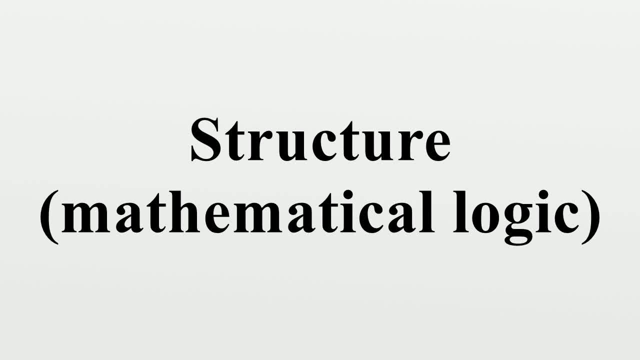 but there is no requirement that it satisfy any of the field axioms. The rational numbers q, the real numbers r and the complex numbers c, like any other field, can be regarded as sigma s Sigma structures in an obvious way, whereas addition of rational numbers is multiplication. 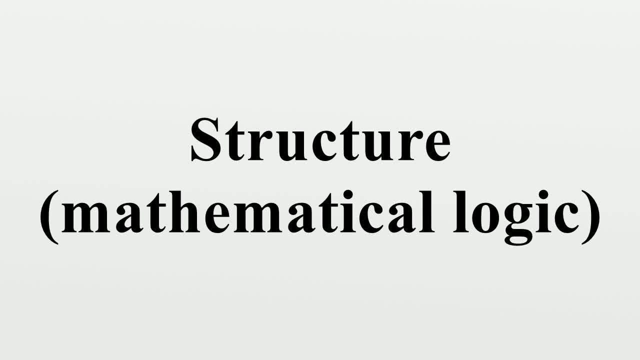 of rational numbers is the function that takes each rational number x to x, and is the number zero and is the number one, and, and are similarly defined. But the ring z of integers, which is not a field, is also a sigma f structure, in the same way, In fact. 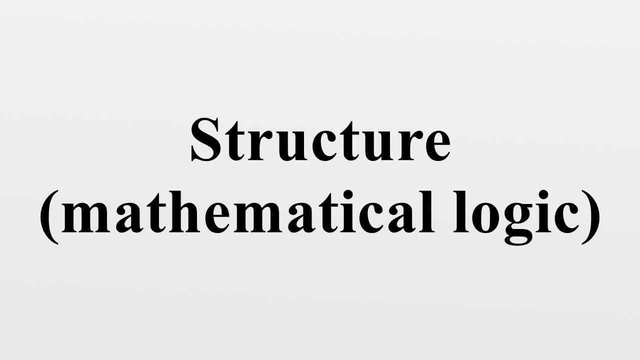 there is no requirement that any of the field axioms hold in a sigma f structure. A signature for order fields needs an additional binary relation, such as less than or, and. therefore structures for such a signature are not algebras, even though they are, of course, algebraic structures. 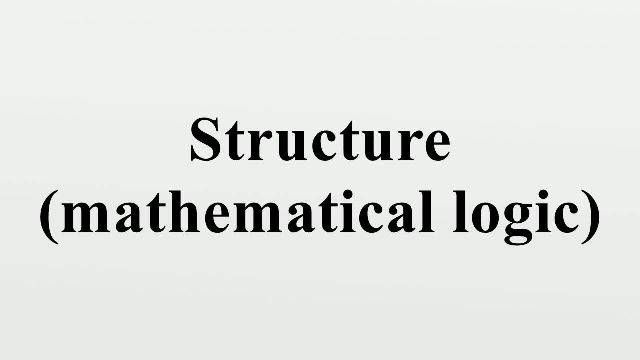 in the usual loose sense of the word. The ordinary signature for set theory includes a single binary relation. A structure for this signature consists of a set of elements and an interpretation of the relation as a binary relation on. these elements Induce substructures and closed subsets. 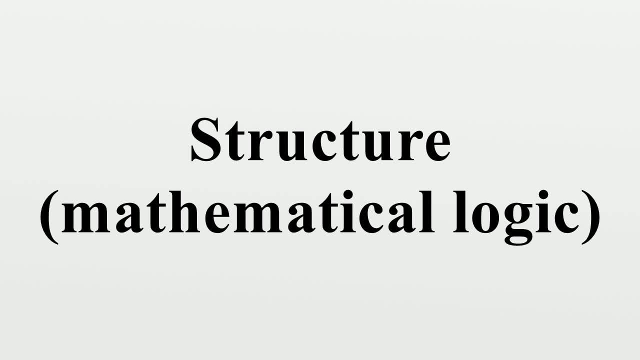 Sets is called an substructure of if and have the same signature. The domain of is contained in the domain of, and the interpretations of all function and relation symbols agree on The usual notation for this relation is a subset of the domain of a structure. 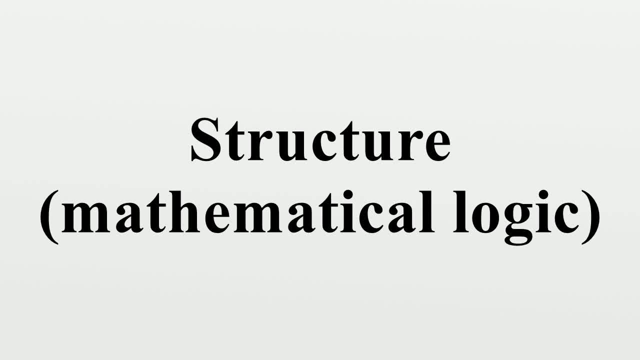 is called closed if it is closed under the functions of ie. if the following condition is satisfied: for every natural number n, every n-a-r-y function symbol f in all elements, The rest of the set of atoms is called closed if the structure is closed under the functions. 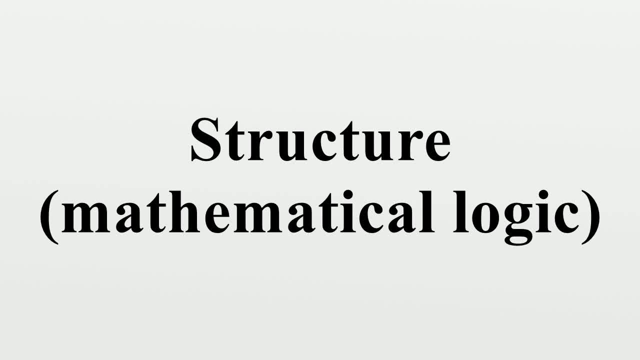 result of applying f to the n-tuple is again an element of B. For every subset there is a smallest closed subset of that contains B. It is called the closed subset generated by B or the hull of B, and denoted by OR. The operator is a. 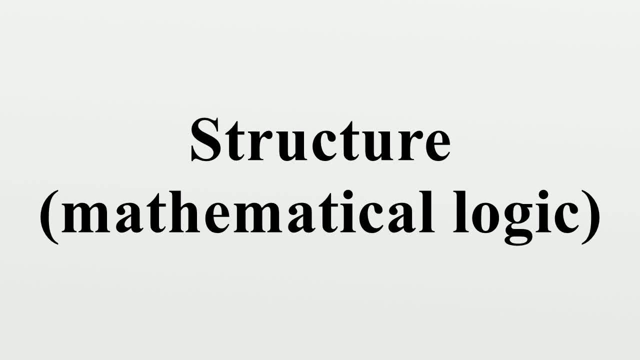 finitary closure operator on the set of subsets SIV. If an is a closed subset, then is an induced substructure of, where assigns to every symbol of sigma the restriction to B of its interpretation in. Conversely, the domain of an induced substructure is a closed subset, The closed subsets of a structure or form: a. 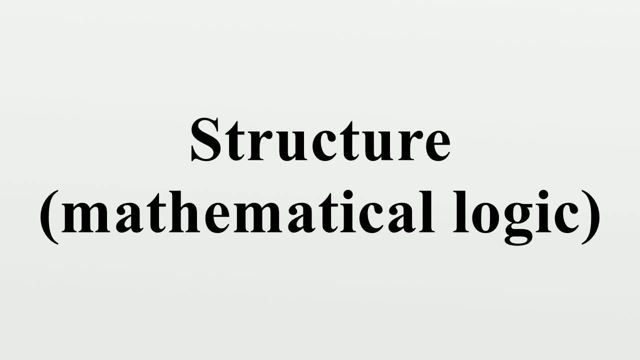 lattice. The meet of two subsets is their intersection. The join of two subsets is the closed subset generated by their union. Universal algebra studies the lattice of substructures of a structure in detail Examples. let sigma equals plus times minus zero. 1. Be again the standard signature for fields When regarded as sigma structures. 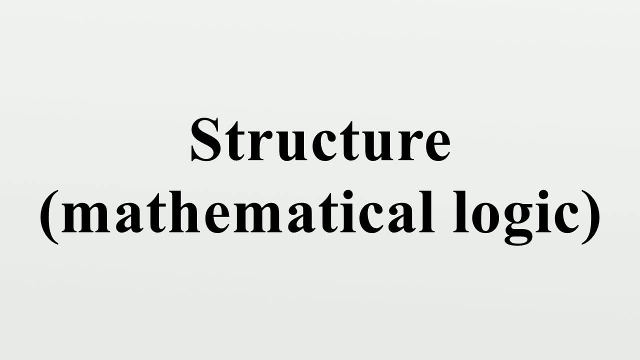 in the natural way. the rational numbers form a substructure of the real numbers and the real numbers form a substructure of the complex numbers. The rational numbers are the smallest substructure of the real numbers. that also satisfies the field axioms. The set of integers gives an even smaller substructure of the real 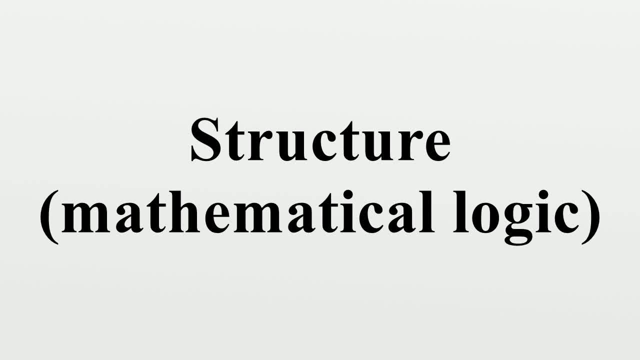 numbers, which is not a field. Indeed, the integers of the real numbers are the substructure of the real numbers generated by the empty set. using this signature, The notion in abstract algebra that corresponds to a substructure of a field in this signature is that of a subring rather than that of a subfield. 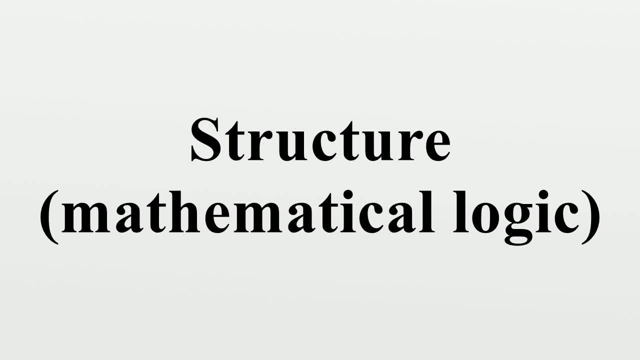 The most obvious way to define a graph is a structure with a signature sigma consisting of a single binary relation, symbol E. The vertices of the graph form the domain of the structure and for two vertices are and be. E means that a and b are connected by an edge. In this encoding the notion of induced 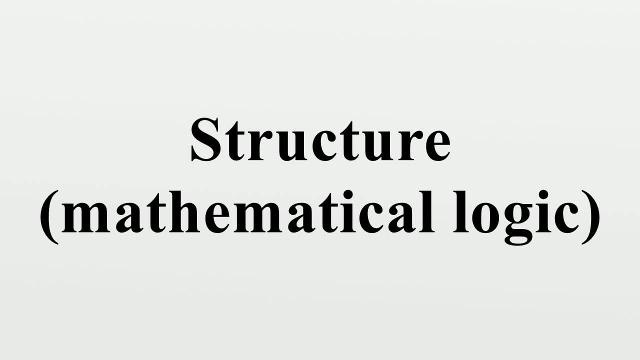 substructure is more restrictive than the notion of subgraph. For example, let G be a graph consisting of two vertices connected by an edge and let H be the graph consisting of the same vertices but no edges. H is a subgraph of G, but not an induced substructure. 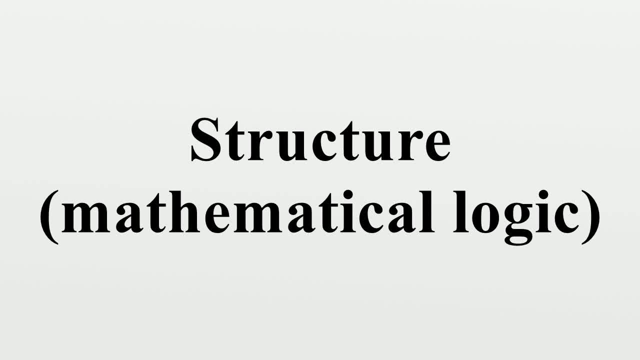 The notion in graph theory that corresponds to induced substructures is that of induced subgraphs, homomorphisms and embeddings. Homomorphisms given two structures and of the same signature sigma. a homomorphism from two is a map that preserves the functions and relations More precisely for every n-a-r-y. 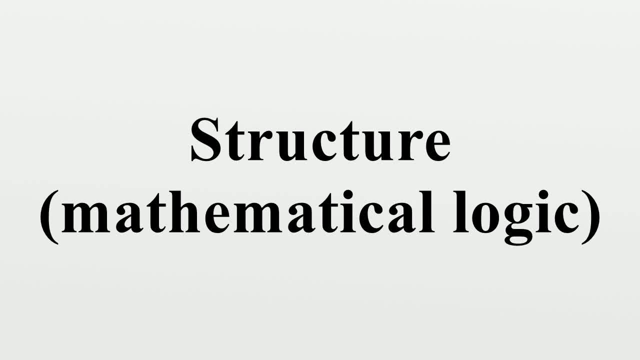 function. symbol f of sigma and any elements. the following equation holds For every n-a-r-y relation. symbol r of sigma and any elements. the following implication holds For a homomorphism h from two is: for every signature sigma, there is a concrete category. 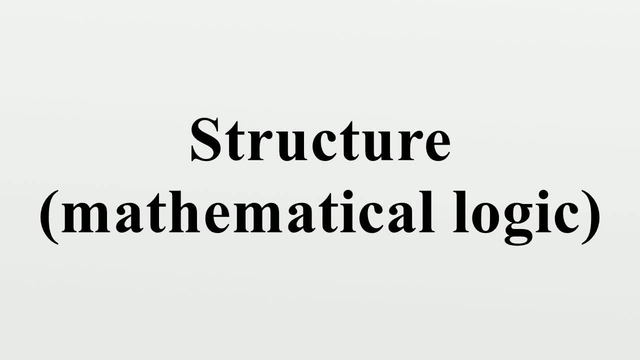 sigma hom, which has sigma structures as objects and sigma homomorphisms as morphisms. A homomorphism is sometimes called strong if for every n-a-r-y relation, symbol r and any elements such that there are such that and the strong homomorphisms give rise to. 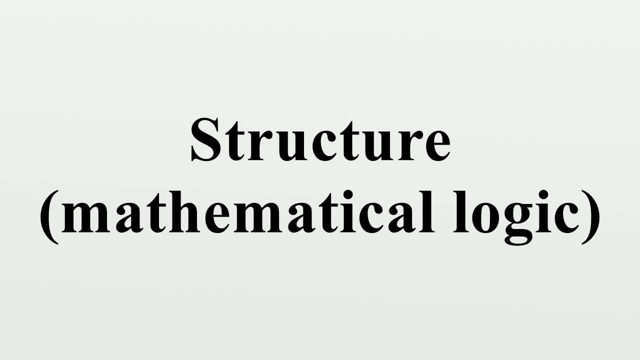 a subcategory of sigma: hom embeddings. A homomorphism is called a embedding if it is one-to-one and for every n-a-r-y relation, symbol r of sigma and any elements, the following equivalence holds: Thus, an embedding is the same thing as a strong homomorphism, which 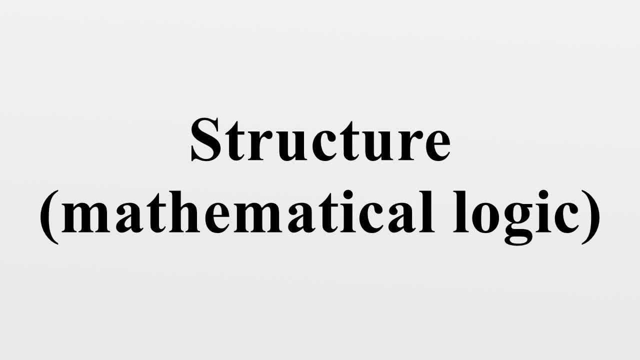 is one-to-one. The category sigma-em-b of sigma structures and sigma embeddings is a concrete subcategory of sigma hom. Induced substructures correspond to subobjects in sigma-em-b. If sigma has only function symbols, sigma-em-b is the subcategory of monomorphisms of σ-HOM. In this case, induced substructures also correspond. 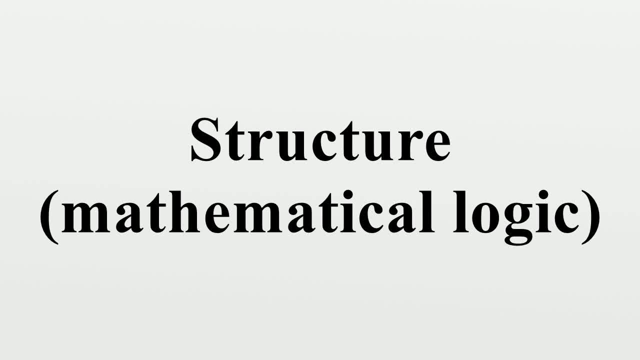 to sub-objects. in σ-HOM Example, as seen above, in the standard encoding of graphs as structures, the induced substructures are precisely the induced subgraphs. However, a homomorphism between graphs is the same thing as a homomorphism between the two structures. 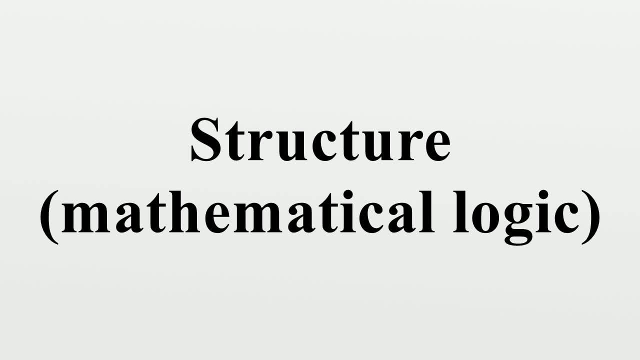 coding the graph. In the example of the previous section, even though the subgraph H of G is not induced, the identity map id HG is a homomorphism. This map is in fact a monomorphism in the category σ-HOM and therefore H is a sub-object of G, which is not an induced substructure. 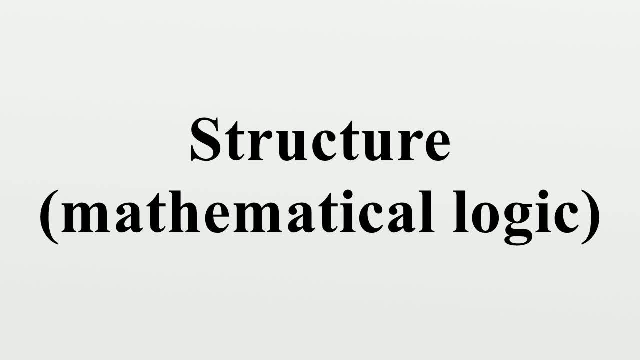 Homomorphism problem. The following problem is known as the homomorphism problem. Given two finite structures and of a finite relational structure signature, find a homomorphism or show that no such homomorphism exists. Every constraint satisfaction problem has a translation into the homomorphism problem. Therefore, the complexity of CSP can be studied using the methods of finite model. 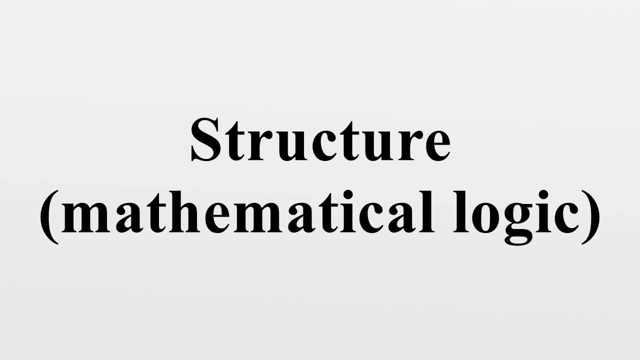 theory. Another application is in database theory, where a relational model of a database is essentially the same thing as a relational structure. It turns out that a conjunctive query on a database can be described by another structure in the same signature as the database model. A homomorphism from the relational model to the structure or representing the query is the 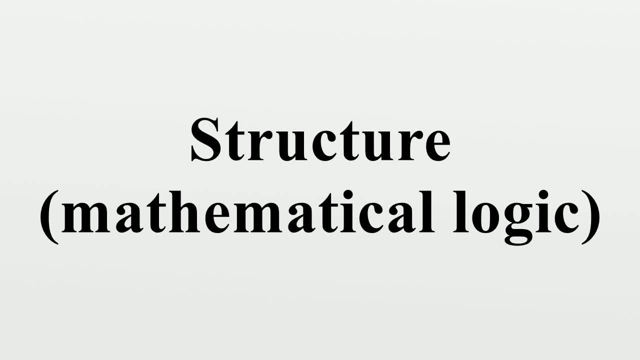 same thing as a solution to the query. This shows that the conjunctive query problem is also equivalent to the homomorphism problem. Structures and first-order logic Structures are sometimes referred to as first-order structures. This is misleading, as nothing in the definition ties them to any specific logic and in fact they are suitable as semantic. 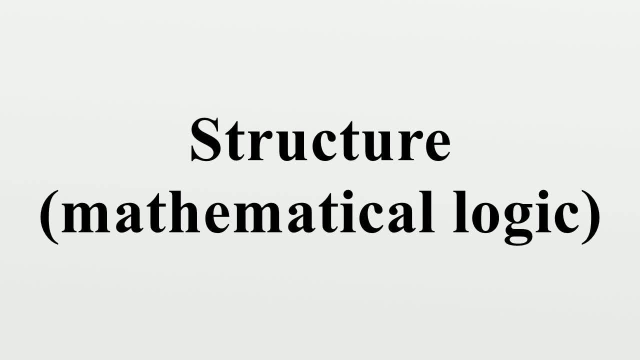 objects, both for very restricted fragments of first-order logic, such as that used in universal algebra, and for second-order logic In connection with first-order logic and model theory. structures are often called models, even when the question models of what has no obvious answer. 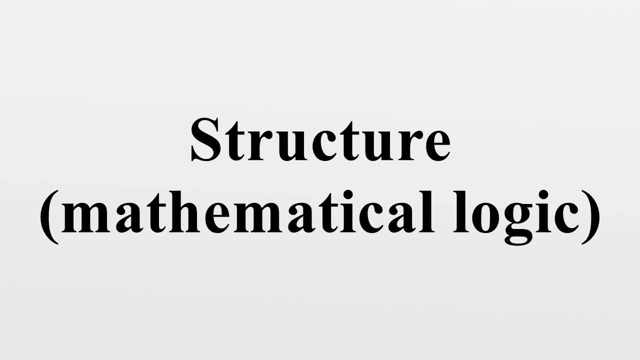 Satisfaction- Satisfaction Relation. Each first-order structure has a satisfaction relation defined for all formulas in the language consisting of the language of, together with a constant symbol for each element of M, which is interpreted as that element. This relation is defined inductively using Tarshi's T-schema. A structure is said to be a model of a theory T if the language of is the same as the language of T and every sentence in T is 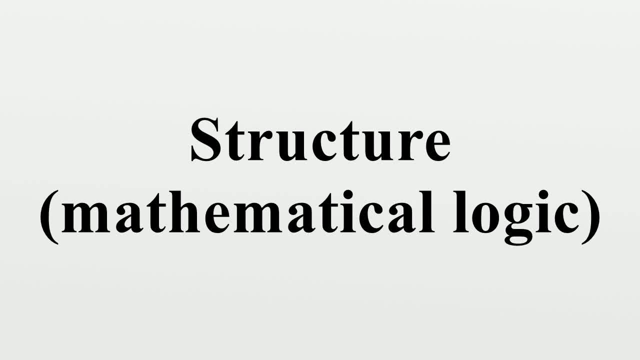 satisfied by. Thus, for example, a ring is a structure for the language of rings that satisfies each of the ring axioms. who Definable relation, an a-r, y related on the universe M of a structure is He said to be the? 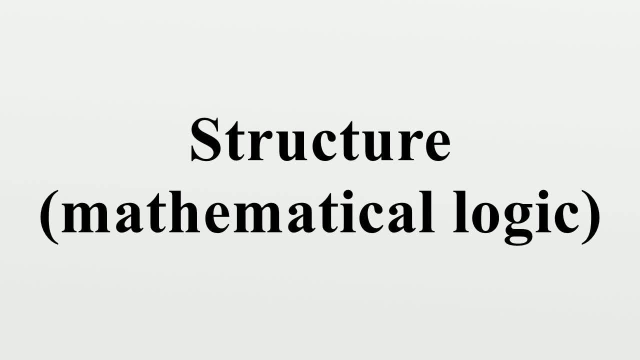 John, there is a formula in such to. it is one somebody if, similar to, if you would. An important special case is the definability of specific elements. An element M of M is definable in if, and only if, there is a formula phi such that definability with parameters A relation R is said to be definable. 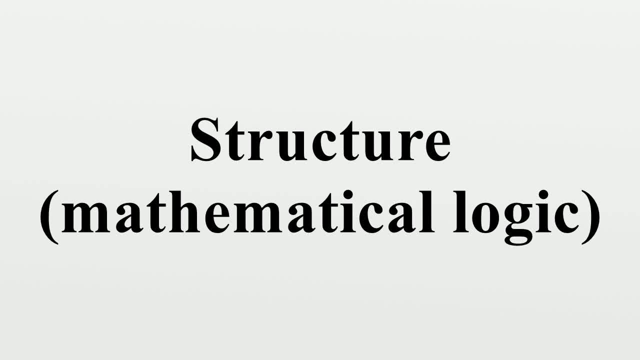 With parameters. if there is a formula phi with parameters from, such that R is definable using phi, Every element of a structure is definable using the element itself as a parameter. It should be noted that some authors use definable to mean definable without parameters, while other authors mean definable with parameters. 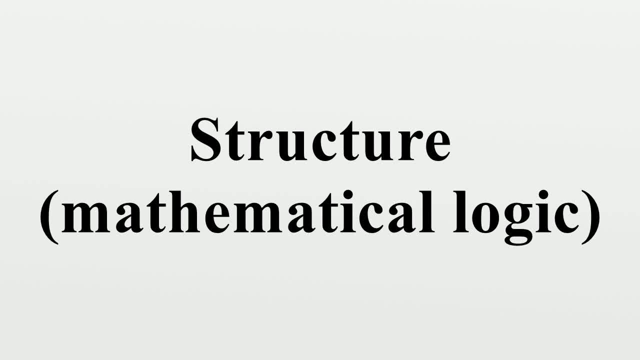 Broadly speaking, the convention that definable means definable without parameters is more common amongst set theorists, while the opposite convention is more common amongst model theorists: Implicit definability. recall from above that an N-A-R-Y relation, R on the universe, M of a structure, is explicitly defined. 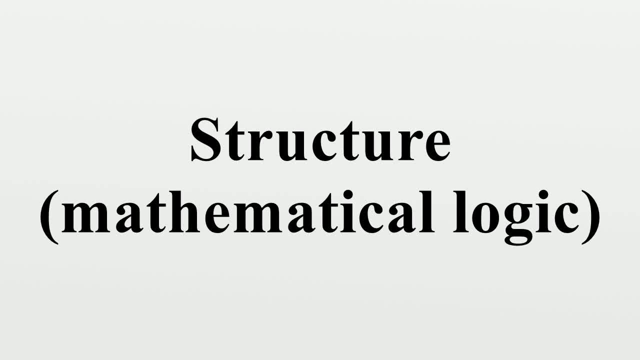 if there is a formula phi, such that here the formula phi used to define a relation, R, must be over the signature of, and so phi may not mention R itself, since R is not in the signature of. if there is a formula phi in the extended language containing the language of an anew symbol, R, 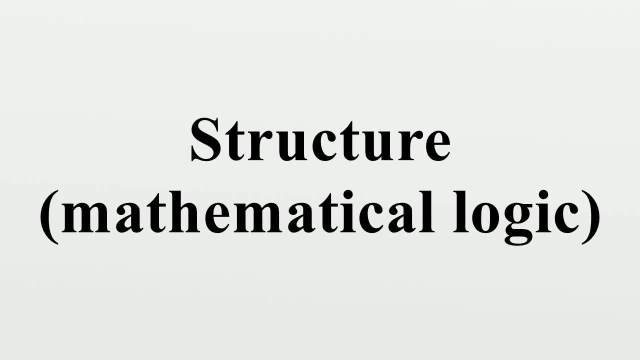 and the relation R is the only relation. on such that, then, R is said to be implicitly definable over by Beth's theorem: every implicitly definable relation, Any relation, is explicitly definable. Many sorted structures, Structures as defined above, are sometimes called one-sorted structures to distinguish them from the more general many-sorted structures. 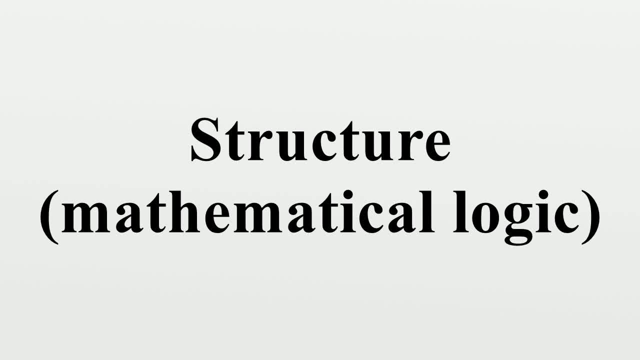 A many-sorted structure can have an arbitrary number of domains. The sorts are part of the signature and they play the role of names for the different domains. Many-sorted signatures also prescribe on which sorts, the functions and relations of a many-sorted structure. 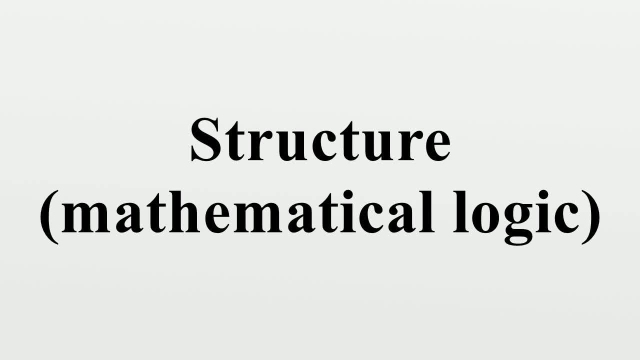 Therefore, the arities of function symbols or relation symbols must be more complicated. objects such as tuples of sorts rather than natural numbers, Vector spaces, for example- can be regarded as two-sorted structures in the following way: The two-sorted signature of vector spaces consists of two sorts- V and S- and the following function symbols: 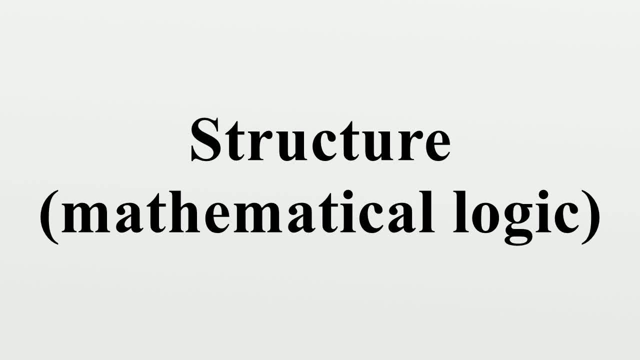 If V is a vector space over a field F, the corresponding two-sorted structure consists of the vector domain, the scalar domain, and the obvious functions such as the vector zero, the scalar zero or scalar multiplication. Many sorted structures are often used as a convenient tool, even when they could be avoided with a little effort. 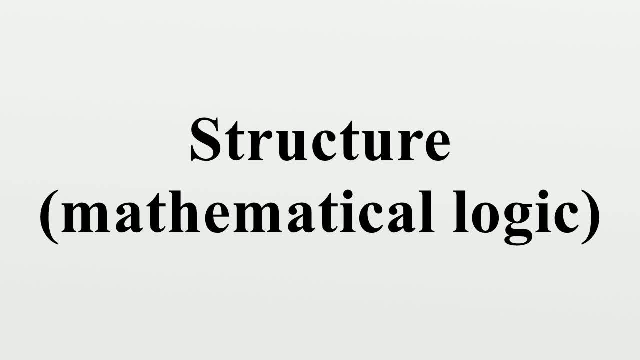 But they are rarely defined in a rigorous way because it is straightforward and tedious to carry out the generalization. In most mathematical endeavors not much attention is paid to the sorts. A many-sorted logic, however, naturally leads to a type theory. As Bart Jacobs puts it, a logic is always a logic over a type theory. 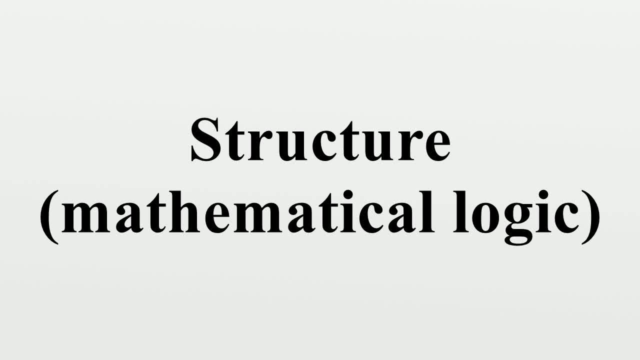 This emphasis in turn leads to categorical logic, because a logic over a type theory categorically corresponds to one category Capturing the logic being fibered over another category capturing the type theory. Other Generalizations: Partial Algebras, Both universal algebra and model theory, study classes of algebras that are defined by a signature and a set of axioms. 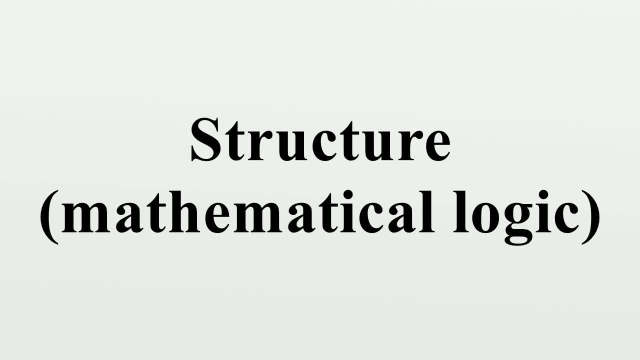 In the case of model theory, these axioms have the form of first-order sentences. The formalism of universal algebra is much more restrictive. Essentially, it only allows first-order sentences that have the form of universally quantified equations. The problem is that there are no equations between terms eg, x, y. 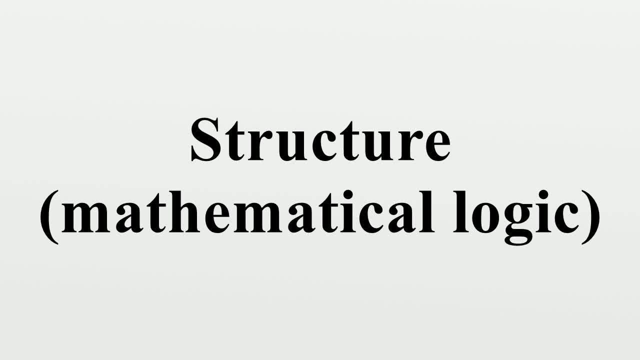 One consequence is that the choice of a signature is more significant in universal algebra than it is in model theory. For example, the class of groups in the signature consisting of the binary function symbol times and the constant symbol 1 is an elementary class, But it is not a variety. 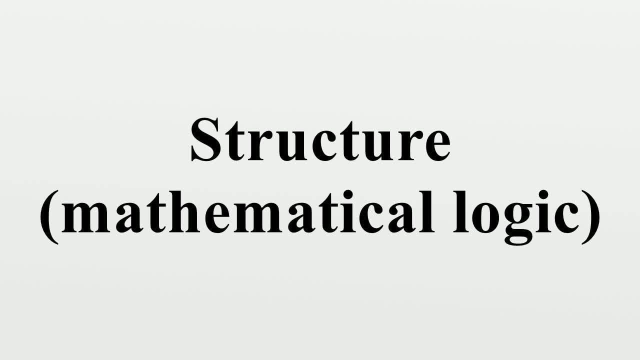 Universal algebra solves this problem by adding a unary function symbol minus 1.. In the case of fields, this strategy works only for addition. For multiplication it fails because 0 does not have a multiplicative inverse. An ad hoc attempt to deal with this would be to define 0-1 equals 0.. 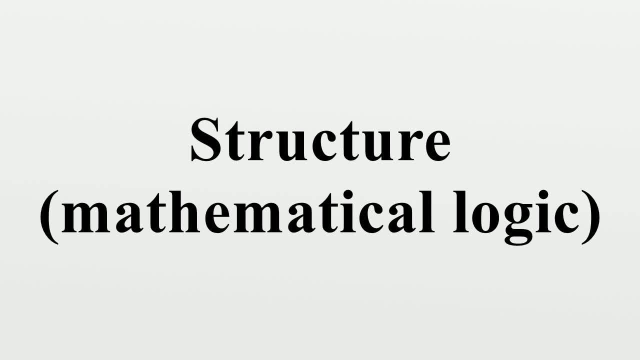 Therefore, 1 is naturally led to allow partial functions, ie functions that are defined only on a subset of their domain. However, there are several obvious ways to generalize notions such as substructure, homogenesis, structure, homomorphism and identity. 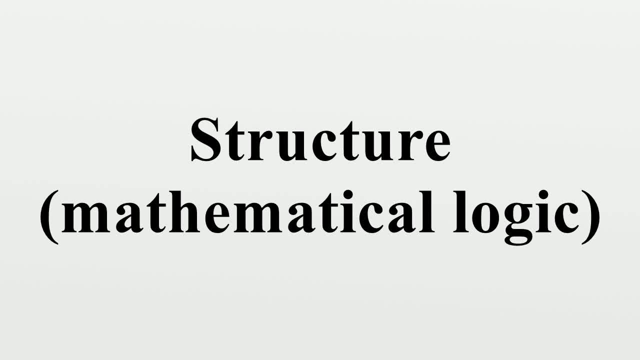 Structures for typed languages. In type theory, there are many sorts of variables, each of which has a type. Types are inductively defined, Given two types: delta and sigma. there is also a type- sigma- delta- that represents functions from objects of type sigma to objects of type delta. 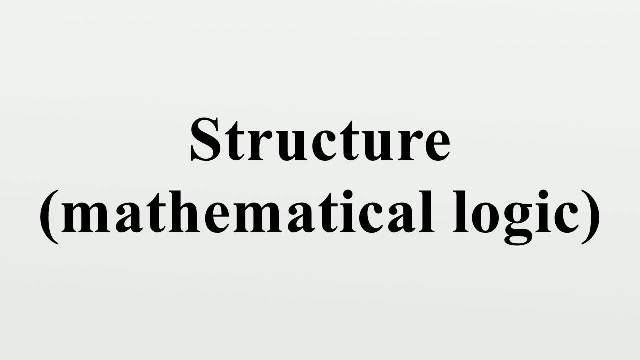 A structure for a typed language must include a separate set of objects of each type And for a function type, The structure must have complete information about the function represented by each object of that type. Higher order languages: There is more than one possible semantics for higher order logic, as discussed in the article on second order logic. 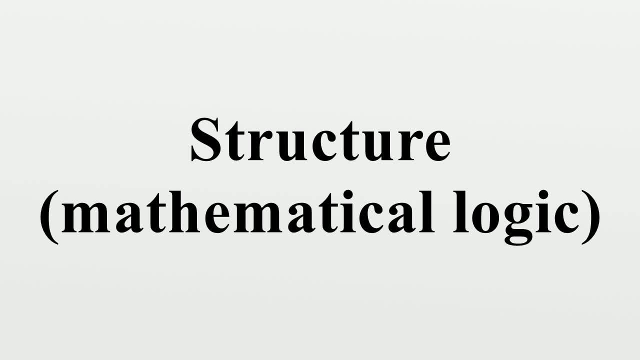 When using full higher order semantics, a structure need only have a universe for objects of type 0. And the T-schema is extended so that a quantifier over a higher order type is satisfied. When using first order semantics, an additional sort is added for each higher order type, as in the case of a many sorted first order language. 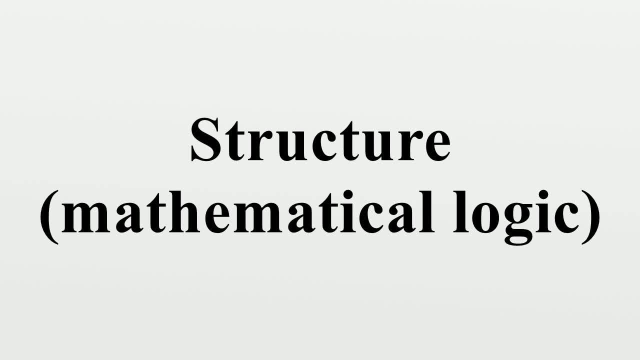 Structures that are proper classes. In the study of set theory and category theory, it is sometimes useful to consider structures in which the domain of discourse is a proper class instead of a set. These structures are sometimes called class models To distinguish them from their set models discussed above. when the domain is a proper class, each function and relation symbol may also be represented by a proper class. 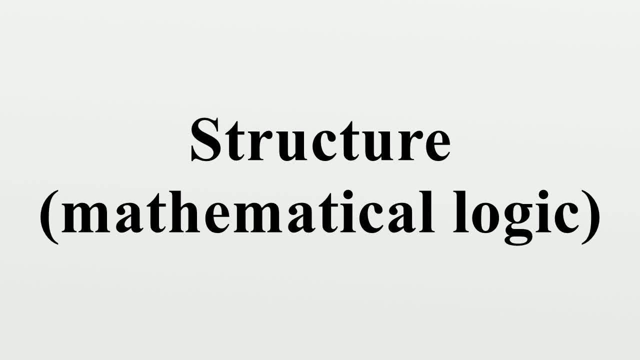 In Bertrand Russell's Principia Mathematica, structures were also allowed to have a proper class as their domain.